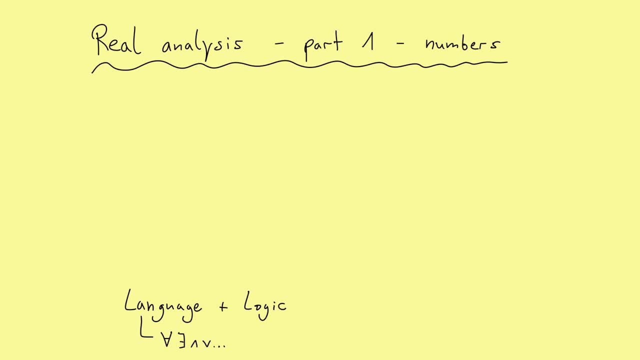 course we need a mathematical logic to give mathematical propositions Meaning to things like a proof. With these two things together we can now formulate some meaningful axioms and then build the whole mathematical building on top of these foundations. Mostly, these axioms are formulated or given in a set theory. 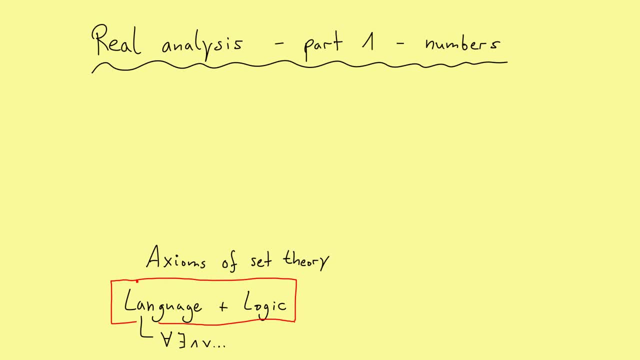 Hence the language, the logic, together with the set theory, gives us the whole mathematical foundation. Now we can build the whole mathematical building on top of our foundation, And often we start with mathematics by introducing the natural numbers. They are given by a set n that consists of the numbers 1, 2, 3, 4 and so on. 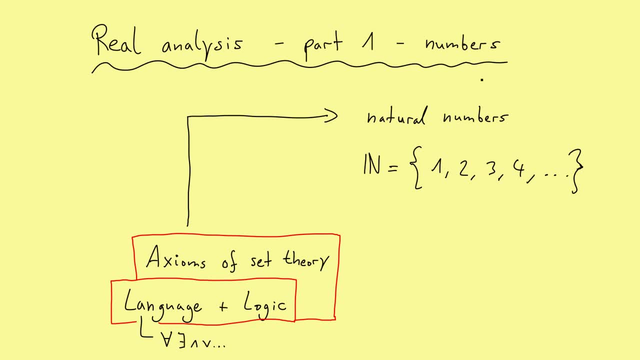 They are natural In the sense that we need them or that they occur in the natural world when we want to count things. There's also an alternative definition for natural numbers when we include 0. So I will call the set n0 and these are the numbers beginning with 0, and then 1,, 2,, 3,, 4 and so on. 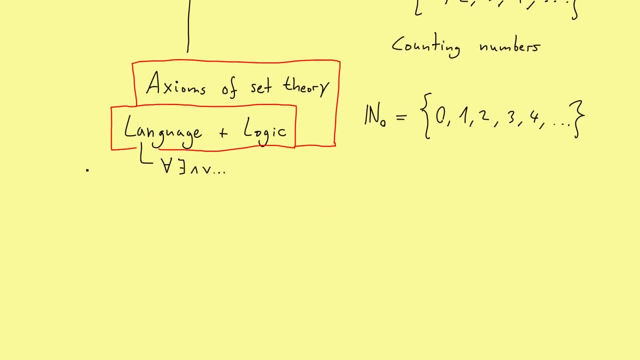 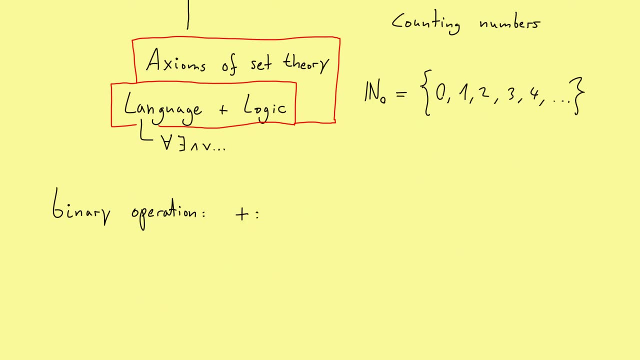 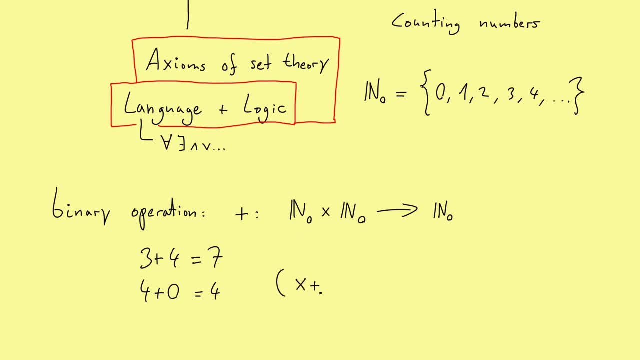 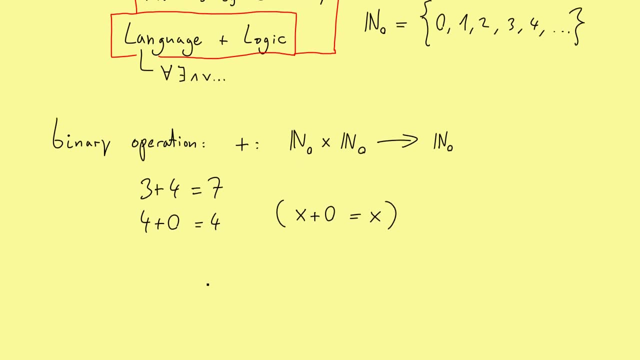 Since 4 plus 0 is 7.. Since 4 plus 0 is 7.. And indeed, every natural number plus zero is the same natural number. Therefore, we call this a neutral element. In mathematics, we call this structure that consists of the set n0 and binary operation. 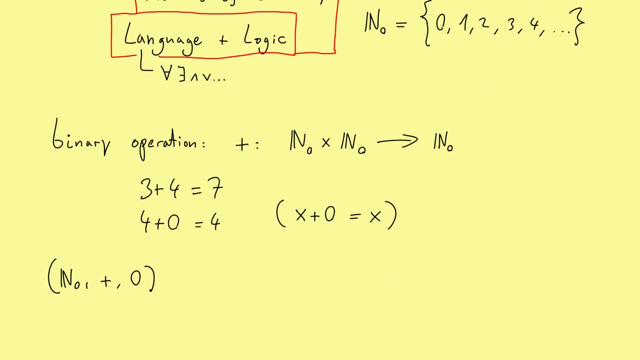 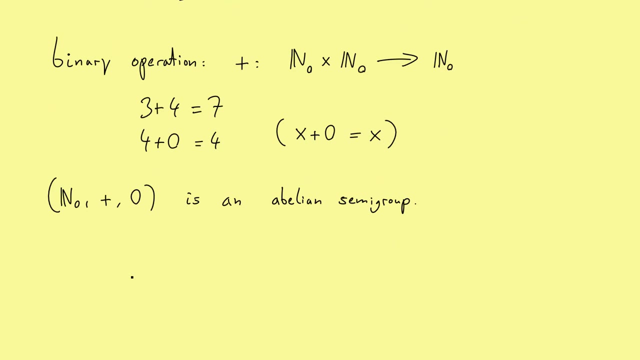 plus and the neutral element 0 and semi-group. And since the plus is commutative, that means the other doesn't matter. we call this an abelian semi-group. What is missing here are the inverses. This means that we don't have an element x that sends 4 to 0.. 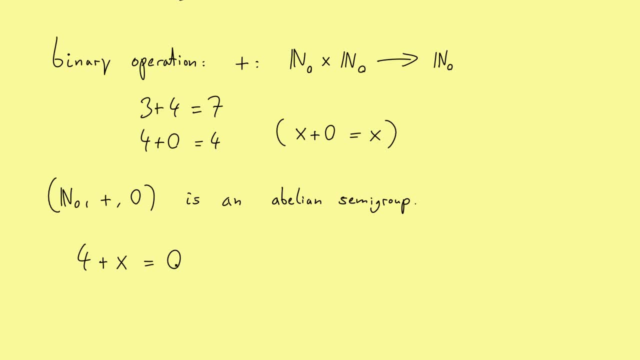 So 4 plus x equals to 0, there is no element x in n or n0 here, Meaning this x would be the inverse of the number 4.. So what we can now do is just adding this inverse in some sense to the set n and n0. 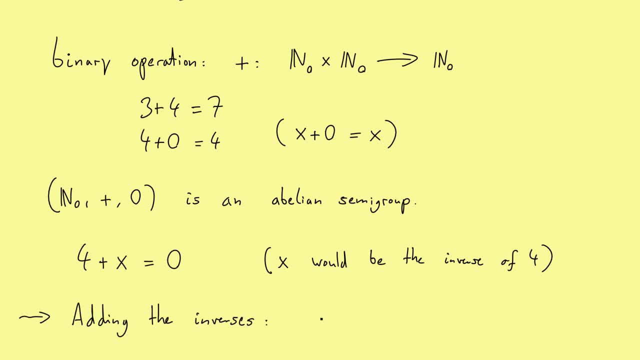 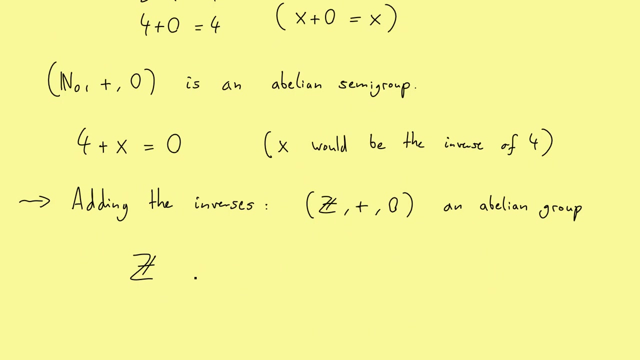 And what we get are the integers. This is now a set z, with plus as the binary operation and the neutral element 0. And since every number has now an inverse, this is what mathematics, in mathematics, is called an abelian group and, as I said before, these numbers are called the integers, the 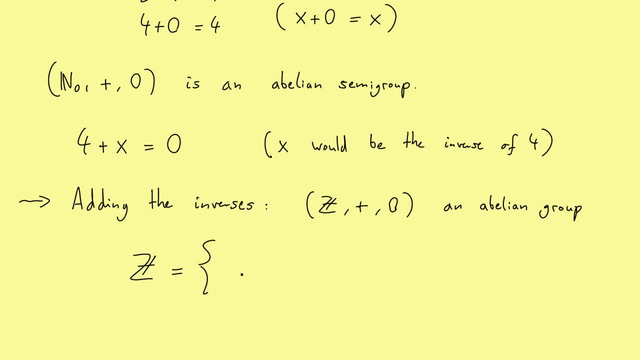 symbol is just the set and the elements. now we can put in with a minus sign, so the inverse of 4 would be called minus 4. of course you know the numbers and we can build them in this sense. and this is the set set and we call the numbers. 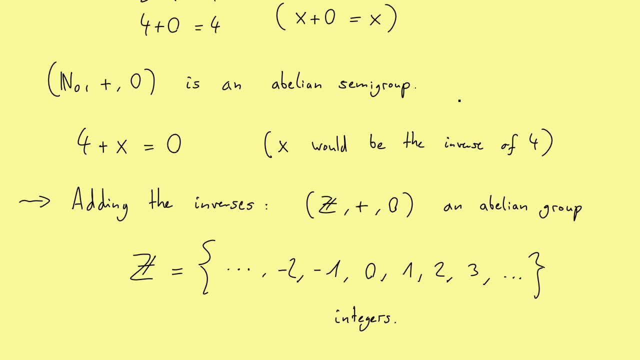 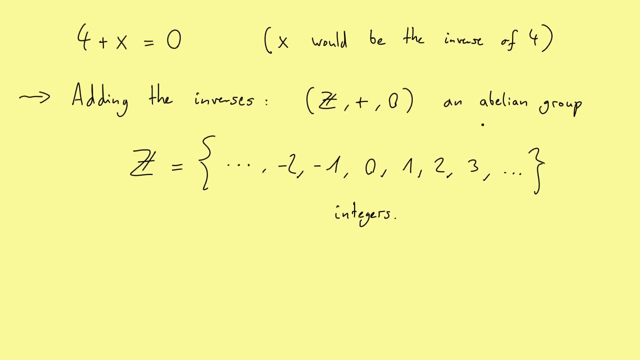 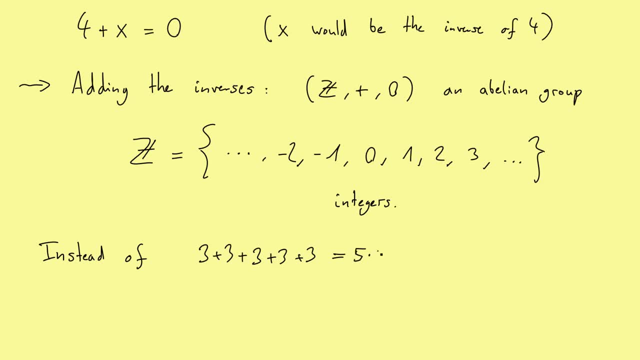 will write, and this 5 times 3. this is shortening the addition, but of course this gives us a new binary operation and we call it the multiplication. again we have the symbol dot, and that goes from times n into the natural numbers n as well. Again, this operation is commutative. 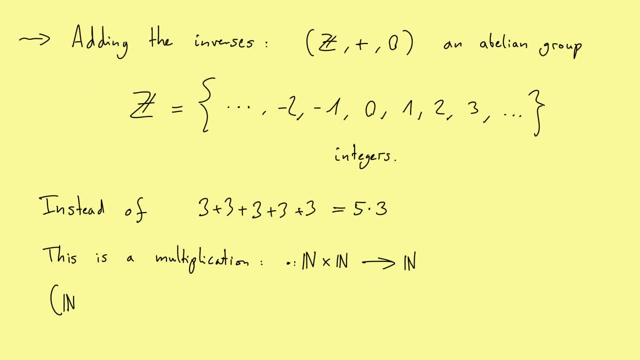 and we get, as mathematicians say, an abelian semi-group, But now with the neutral element 1.. And of course we have to exclude 0 at this point. Without 0, the natural numbers with the multiplication are again an abelian semi-group. And we can do now the same things we did before: we add inverses in. 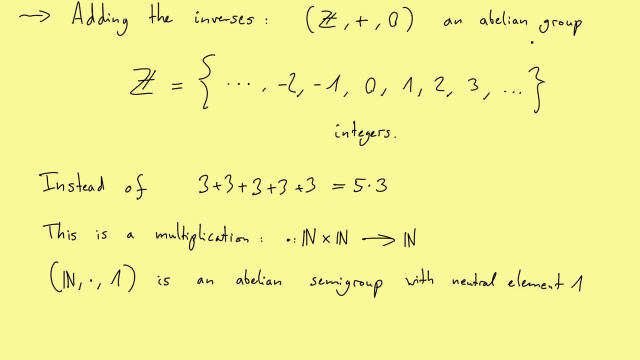 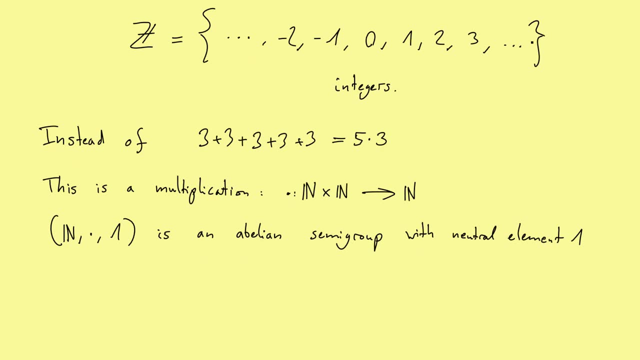 some sense. Of course, I could do this in a formal way, and I have a video about this, But at this point it's just good to know that we can do it and we get again a new structure in mathematics, And this is again an abelian group. Now, every 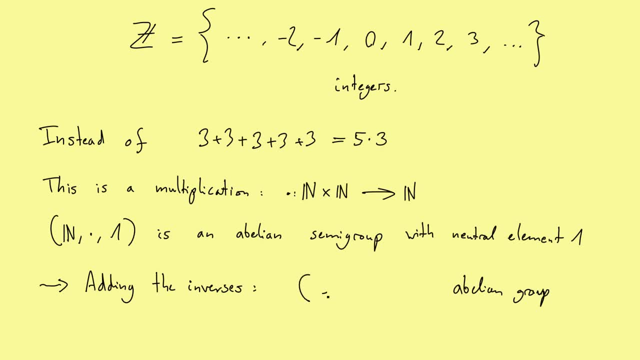 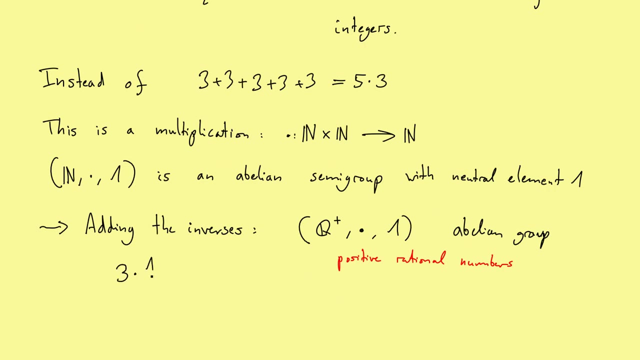 element has an inverse, And these are the rational numbers, The positive rational numbers, to be precise. Of course, this is the same idea as before. I have a natural number 3, for example, But I don't have an element x. that sends this to the. 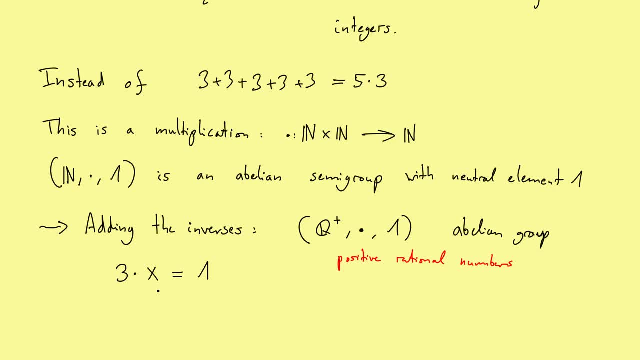 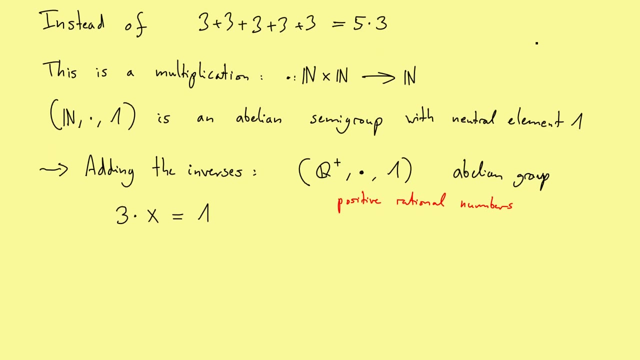 neutral element 1.. Of course this element would be 1 over 3, one-third, But this is not a natural number. We have to add it to the set And then we get the whole set of the positive rational numbers, Putting these together. So add the negative numbers and the 0. We get the. 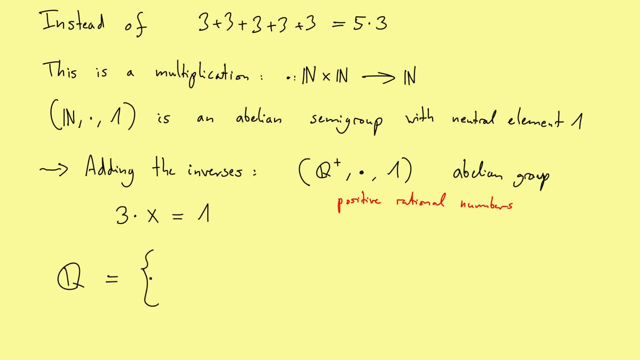 whole set of the rational numbers, And I give this the name q, And the set consists of p over q, So the fractions where p and q are integers, And this is what we call rational numbers. And these rational numbers lie on a number line. This means that we can put each rational 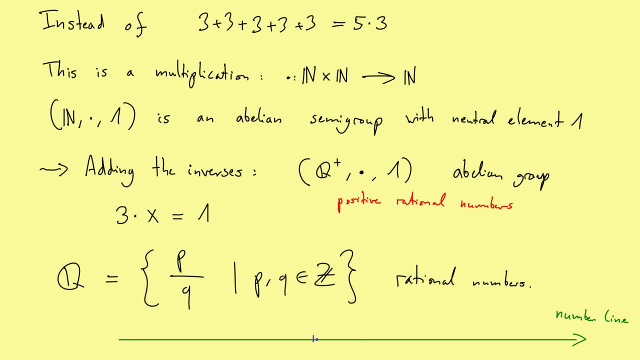 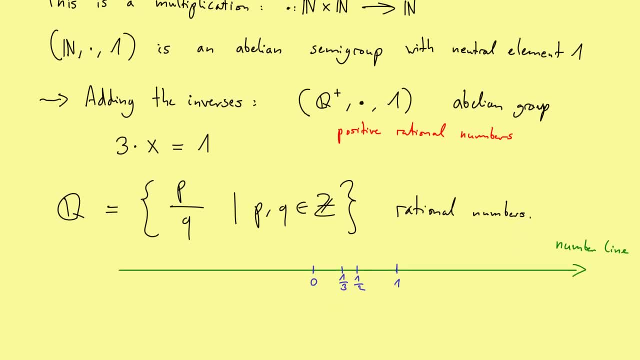 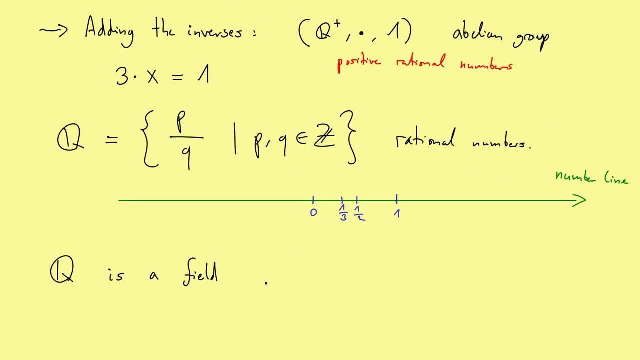 And between there would be one-third, And so on. In mathematics, these rational numbers build a so-called field. This means that we now have two operations that fit together, And these two operations are, of course, addition and multiplication. So, for example, adding two rational numbers is simply given. so 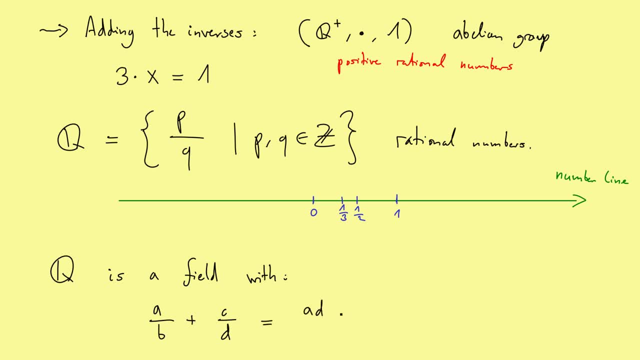 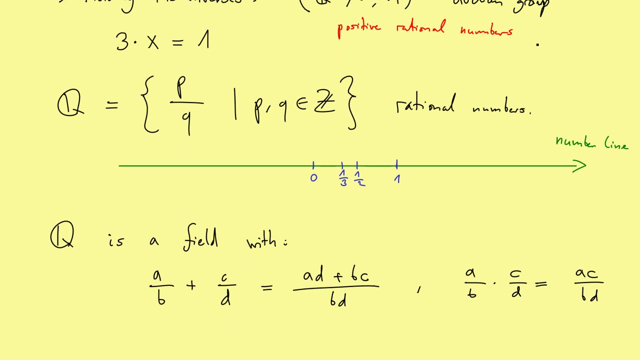 we have the fractions And it is simply given by having same denominator here. So this would be: addition and multiplication is simply easier, just multiplicate denominator and nominator. So ac, bd, And also, as the number line suggests, we have an ordering of the rational numbers, Simply put the: 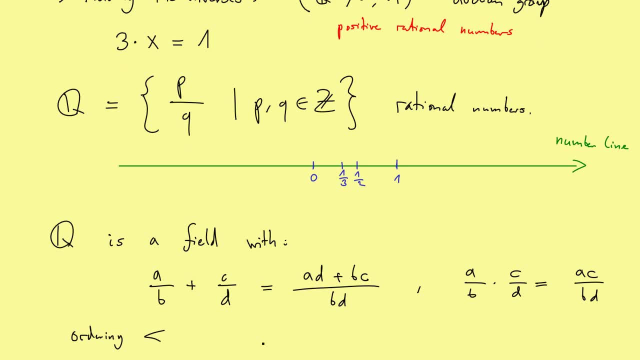 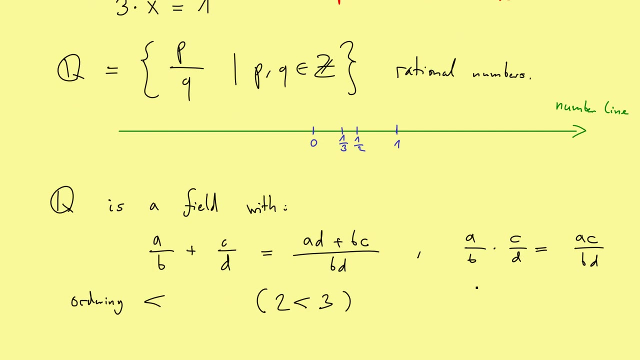 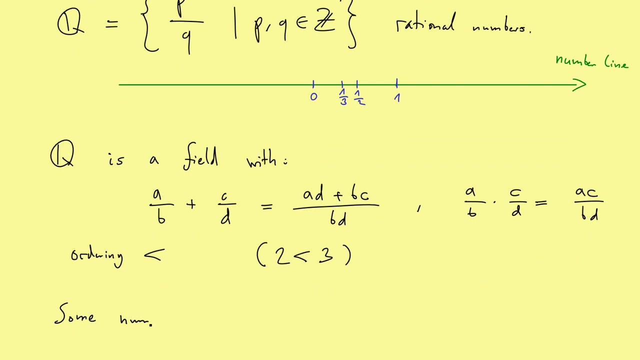 greater sign or the less sign. here, For example, two is less than three. The rational numbers build this field and with the algebraic addition and multiplication we can do a lot of computations. However, it is interesting to know that some numbers are missing on the number line. It is not so clear where. 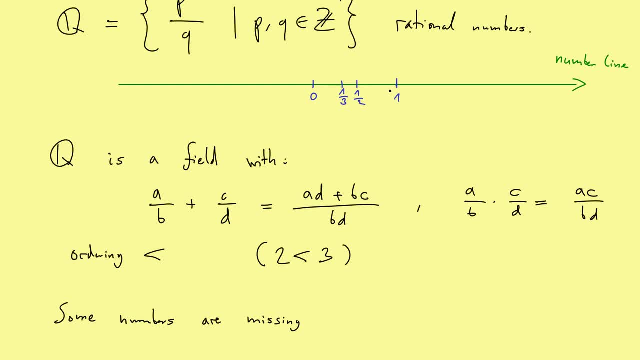 the numbers are missing. It is not so clear where the numbers are missing on the number line. It is not so clear where the numbers are missing on the number line. It is not so clear where these numbers should lie on the number line. but filling in these missing